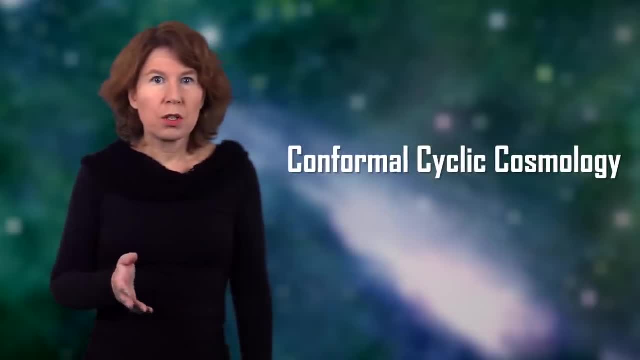 What does CCC mean? I think we're all good with the word cosmology. It's a theory for the history of the entire universe. alright, That it's cyclic means it repeats in some sense. Penrose calls these cycles eons. Each starts with a big bang, but it doesn't end with a big 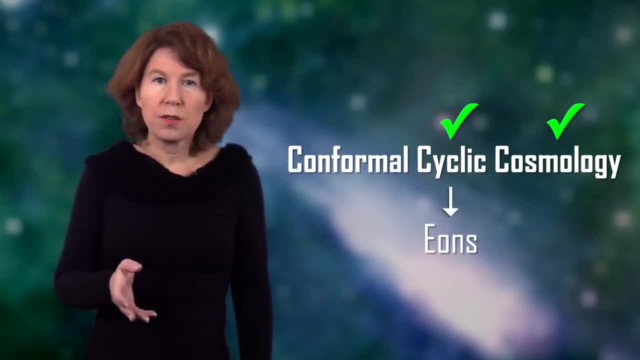 crunch. A big crunch would happen when the expansion of the universe changes to a contraction and eventually all the matter is well crunched together. A big crunch is like a big bang in the universe. This does not happen in conformal cyclic cosmology. Rather, the history of the 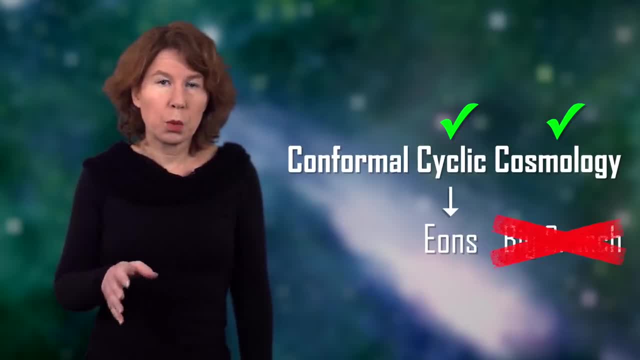 universe just kind of tapers out. Matter becomes more and more thinly diluted. And then there's the word conformal. We need that to get from the thinly diluted end of one eon to the beginning of the next. But what does conformal mean? 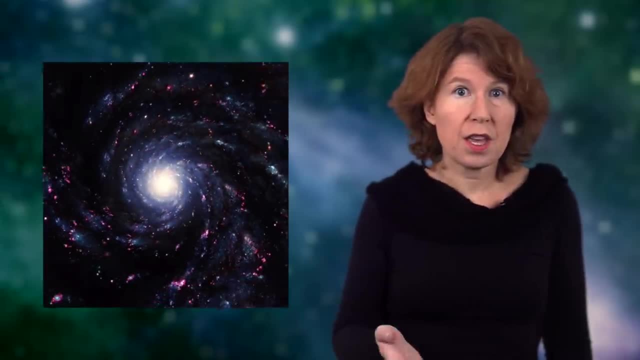 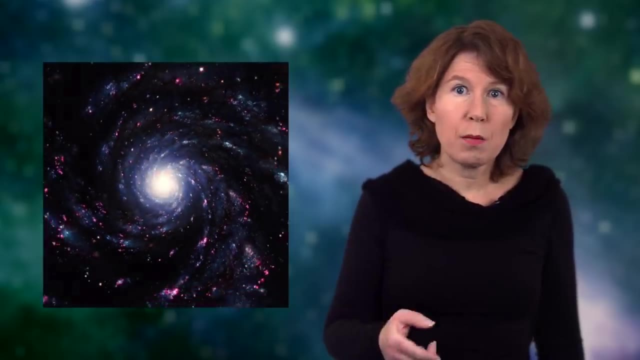 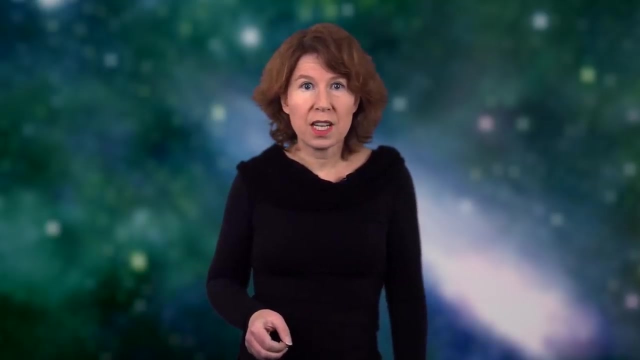 A conformal rescaling is a stretching or shrinking that maintains all relative angles. Penrose uses that because it's the way of life, But because you can use a conformal rescaling to make something that has infinite size into something that has finite size. Here is a simple example of a conformal rescaling. 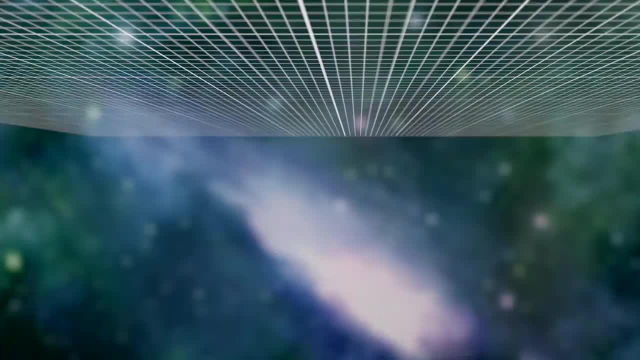 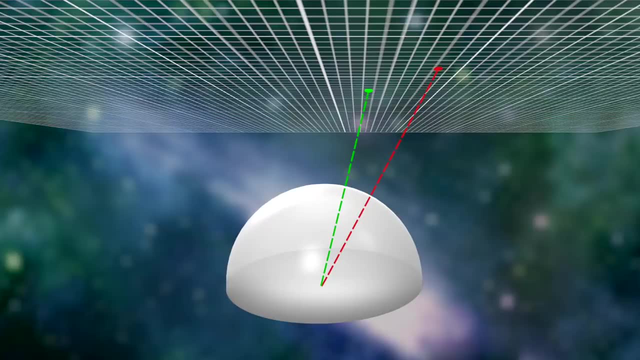 Suppose you have an infinite two-dimensional plane and suppose you have half of a sphere. Now, from every point on the infinite plane you draw a line to the center of the sphere, At the point where it pierces the sphere. you project that down onto a disk. 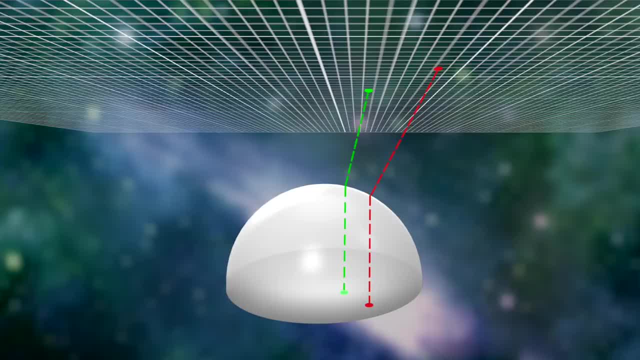 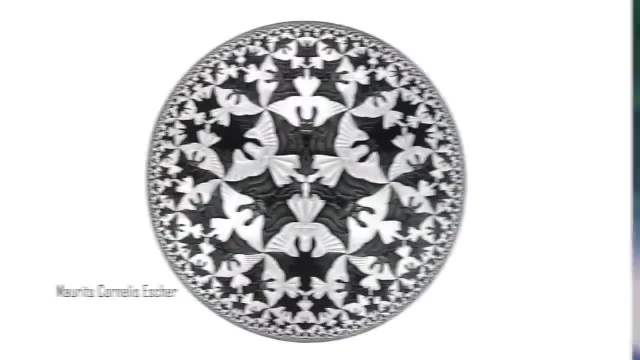 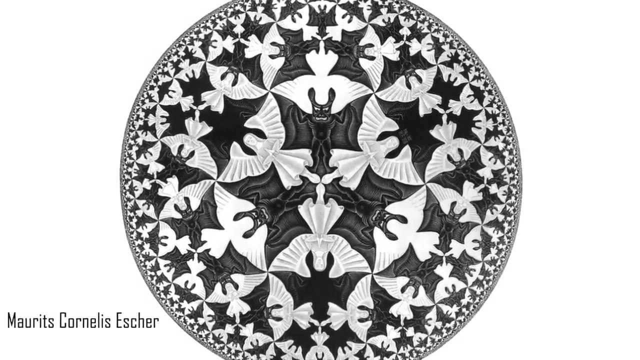 That way you map every point of the infinite plane into the disk underneath the sphere. A famous example of a conformal rescaling is this image from Escher: Imagine that those beds are all the same size and once filled an infinite plane. In this image they are all squeezed into a finite area. Now, in Penrose's case, the infinite thing that you rescale is not just space but space-time. You rescale them both and then you glue the end of our universe to a new beginning. Mathematically you can totally do that. 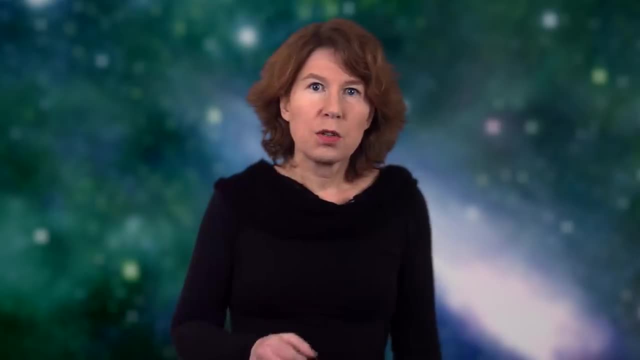 But why would you? And what's with the physics? Let's first talk about why you would want to do that. Penrose is trying to solve a big puzzle in our current theories for the universe: It's the second law of thermodynamics. 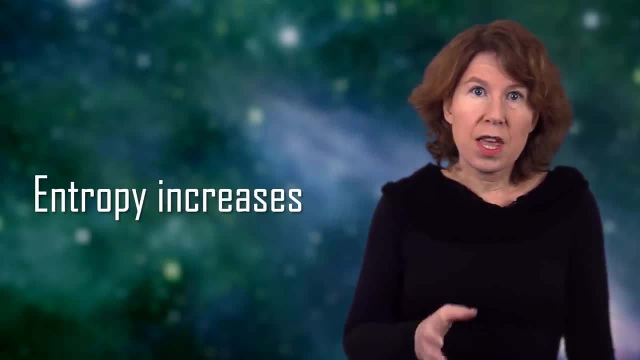 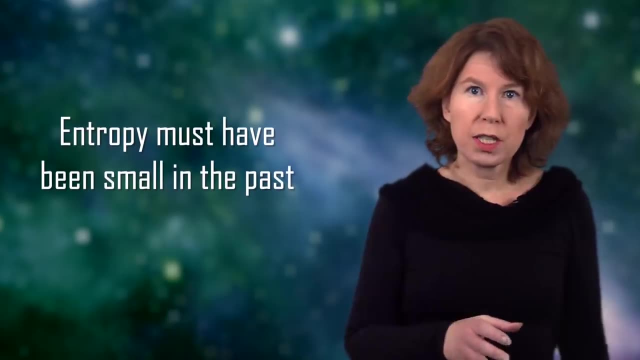 Entropy increases. We see it increase, But that entropy increases means it must have been smaller in the past. Indeed, the universe must have started out with very small entropy. otherwise we just can't explain what we see. That the early universe must have had small entropy is often called the past hypothesis. 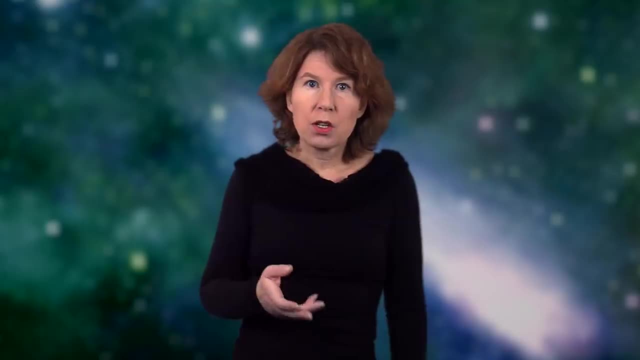 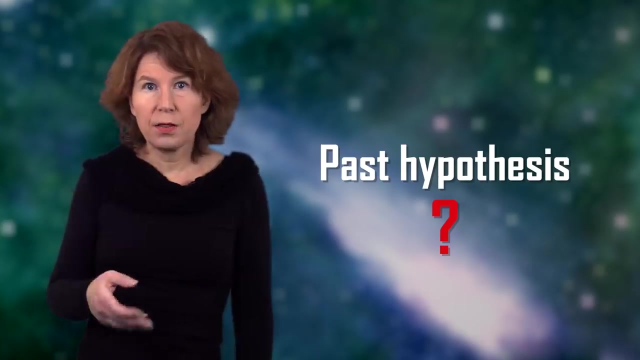 a term coined by the philosopher David Albert. Our current theories work perfectly fine with the past hypothesis, But of course it would be better if one didn't need it, if one instead had a theory from which one could derive it. Penrose has attacked this problem by first finding out that the universe is smaller than 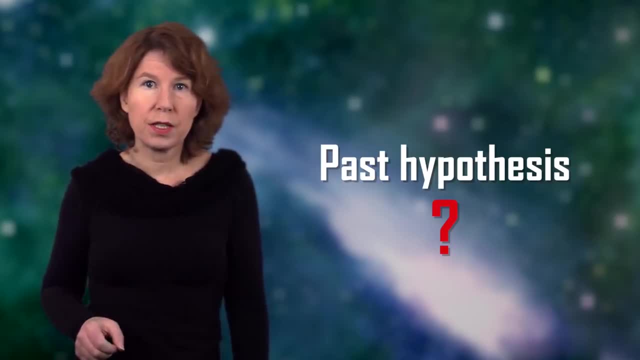 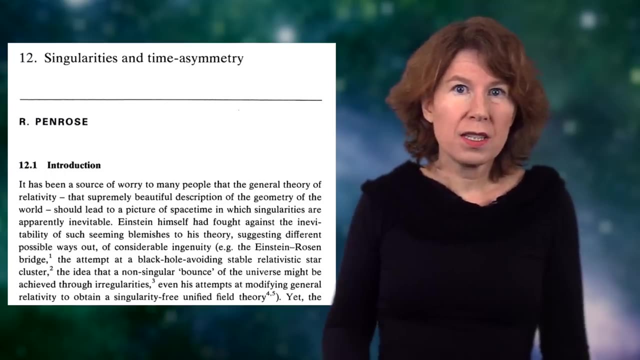 the past And by finding a way to quantify the entropy in the gravitational field. He argued already in the 1970s that it's encoded in the Weyl curvature tensor. That's, loosely speaking, part of the complete curvature tensor of spacetime. 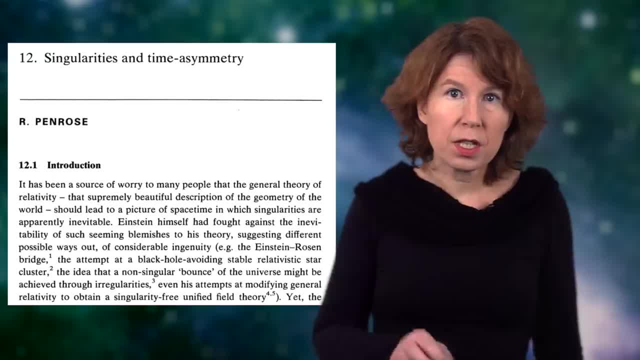 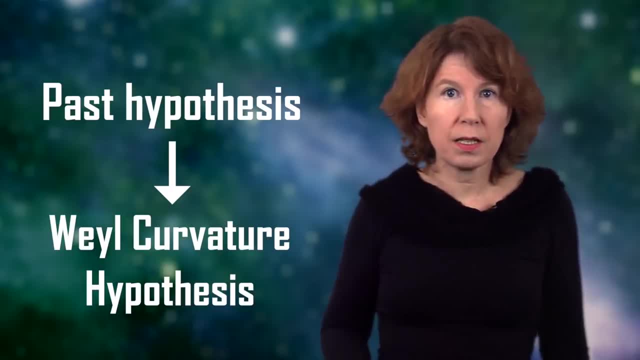 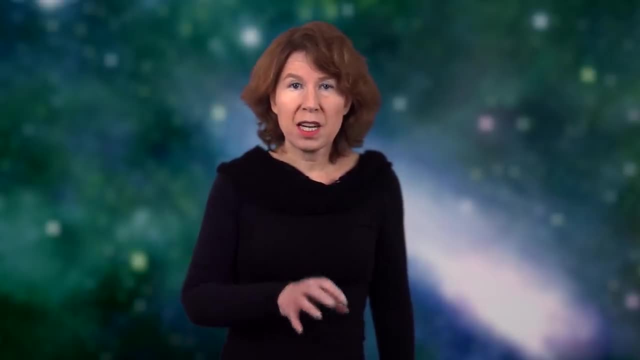 This Weyl curvature tensor, according to Penrose, should be very small in the beginning of the universe. Then the entropy would be small and the past hypothesis would be explained. He calls this the Weyl curvature hypothesis. So instead of the rather vague past hypothesis we now have a mathematically precise Weyl curvature. 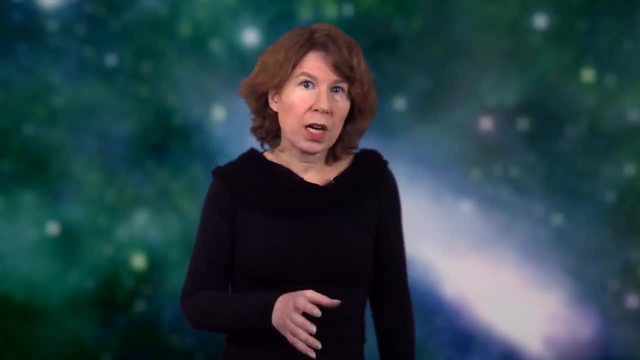 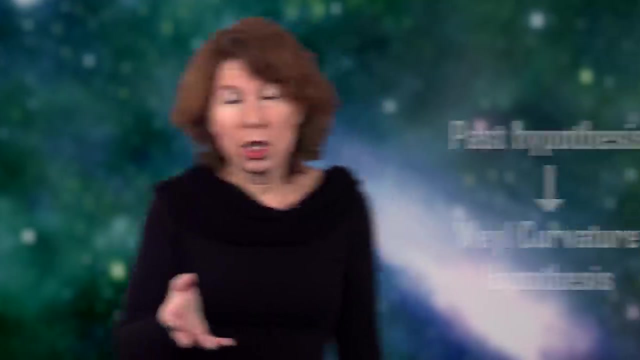 hypothesis, Like the entropy, the Weyl curvature would start initially very small and then increase as the universe gets older. This goes along with the formation of bigger structures like stars and galaxies. Remains the question: how do you get the Weyl curvature to be small? 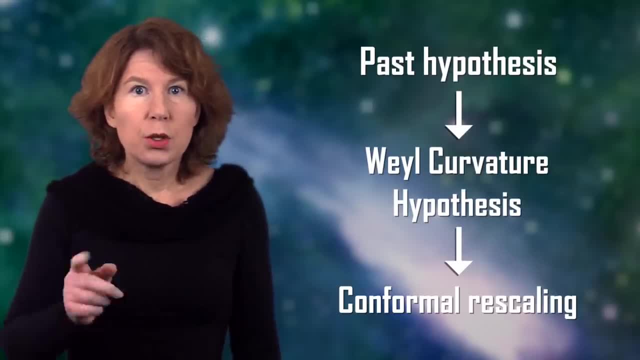 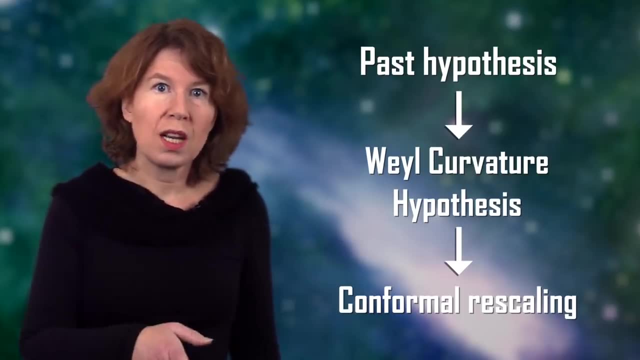 Here's where the conformal rescaling kicks in. You take the end of a universe where the Weyl curvature is large, you rescale it, which makes it very small, and then you postulate that this is the beginning of a new universe. 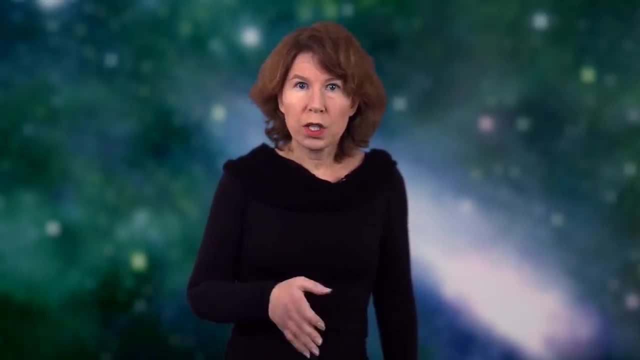 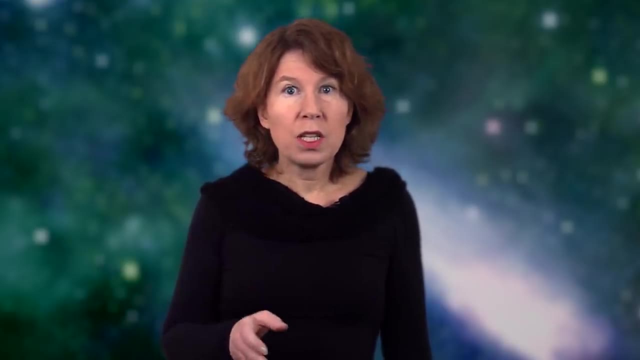 Ok, so that explains why you may want to do that, But what's with the physics? The reason why this rescaling works mathematically is that in a conformally invariant universe there's no meaningful way to talk about time. It's like if I show you a piece of the Koch snowflake and I show you a piece of the Weyl. 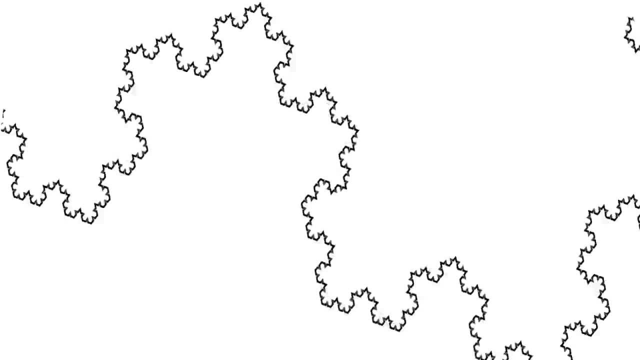 curvature. It's like if I show you a piece of the Koch snowflake and I show you a piece of the Weyl, You ask if that's big or small. These pieces repeat infinitely often so you can't tell if it's big or small. 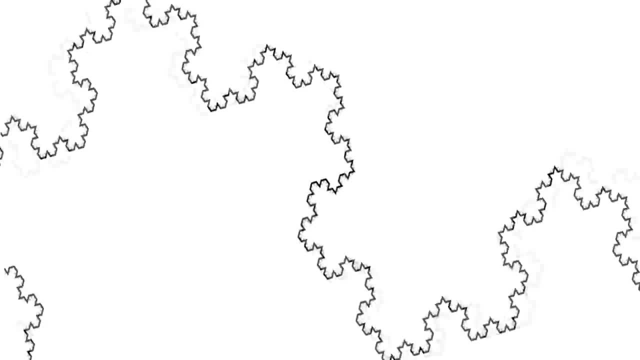 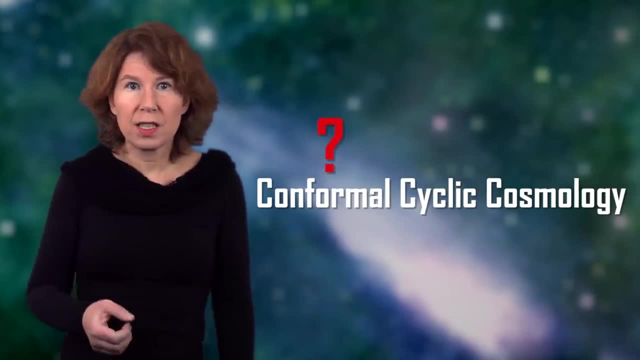 In CCC it's the same with time at the end of the universe, But the conformal rescaling and gluing only works if the universe approaches conformal invariance towards the end of its life. This may or may not be the case. The universe contains massive particles, and massive particles are not conformally invariant. That's because particles are also waves. Massive particles are waves with a particular wavelength, that's the Compton wavelength, which is inversely proportional to the mass. This is a specific scale. so if you rescale the universe, it will not remain the same. However, the masses of the elementary particles all come from the Higgs field. So if you can somehow get rid of the Higgs at the end of the universe, then that would be conformally invariant and everything would work. Or maybe you can think of some other way to get rid of massive particles. 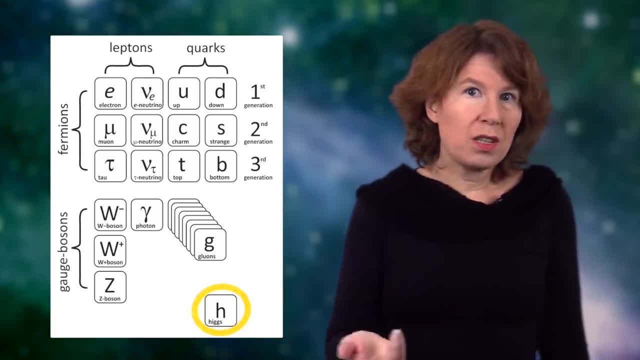 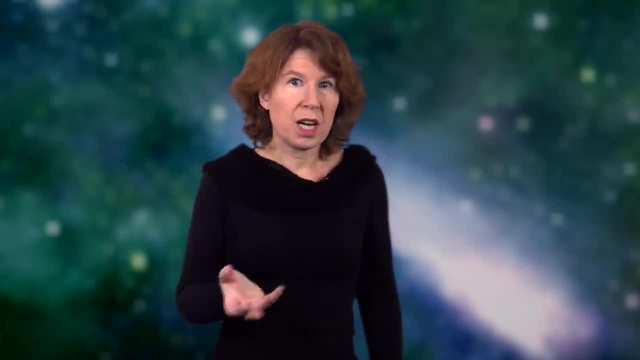 I don't know, And since no one really knows what may happen at the end of the universe, anyway, okay. well, maybe it works somehow, But we can't test what will happen in a hundred billion years. So how could one test Penrose's cyclic cosmology? 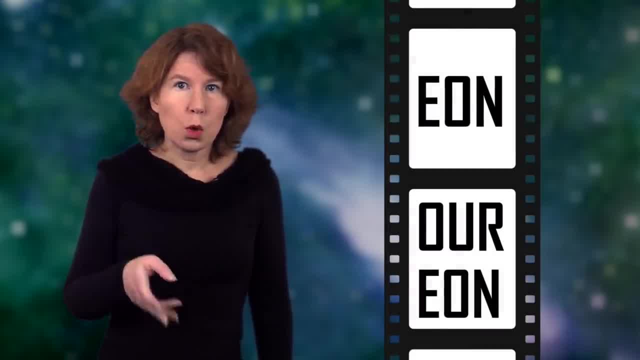 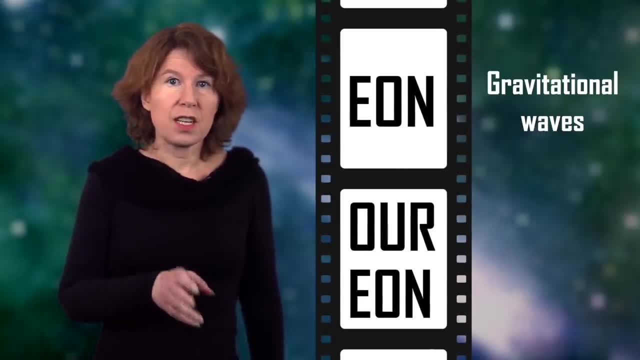 Interestingly, this conformal rescaling doesn't wash out all the details from the previous eon. Gravitational waves survive because they scale differently than the Weyl curvature And those gravitational waves form more or less the same size. The waves from the previous eon affect how matter moves after the big bang of our eon. 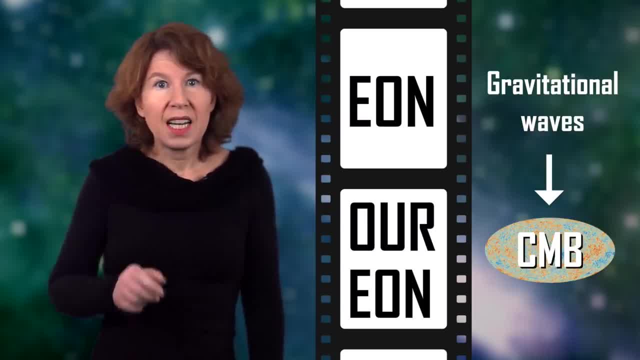 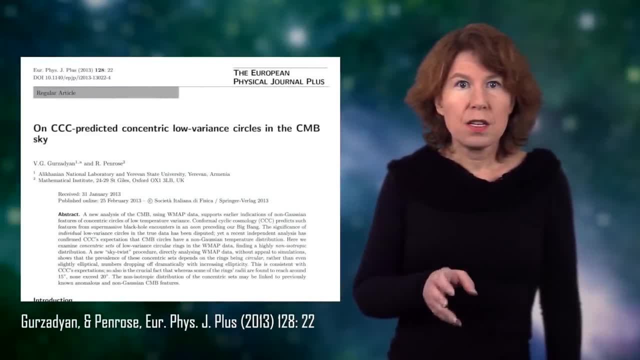 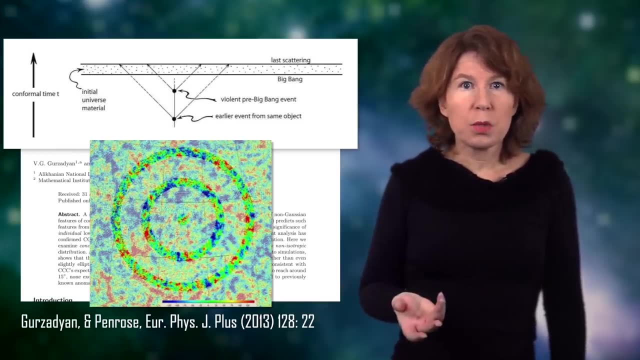 which in turn leaves patterns in the cosmic microwave background, Indeed rather specific patterns. Roger Penrose first said one should look for rings. These rings would come from the collision of supermassive black holes in the eon before ours. This is pretty much the most violent event one can think of, and so it should produce. 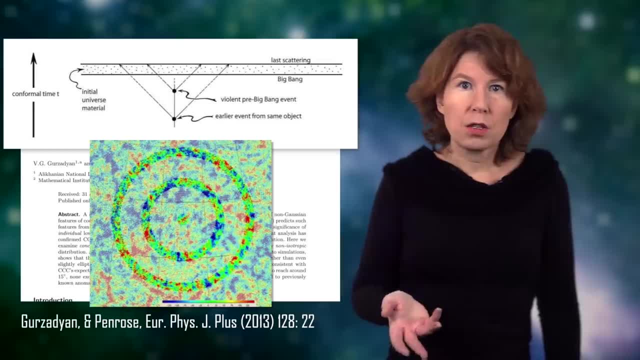 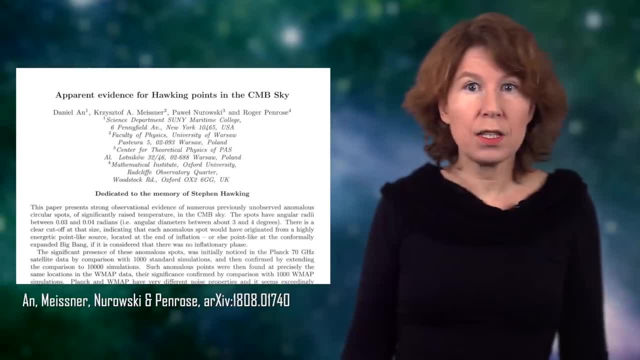 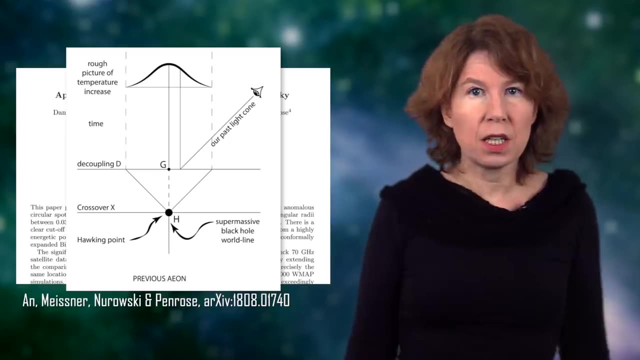 a lot of gravitational waves. However, the search for those signals remained inconclusive. Penrose then found a better observational signature from the earlier eon, which he called Hawking points. Supermassive black holes in the earlier eon evaporate and leave behind a cloud of Hawking. 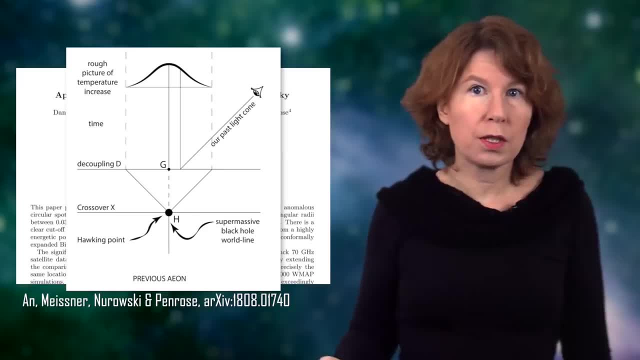 radiation which spreads out over the whole universe. But at the end of the eon you do the rescaling and you squeeze all that Hawking radiation together That carries over into the next eon. So what does that mean? Well, it means that the Hawking points are in the eon and makes a localized point with 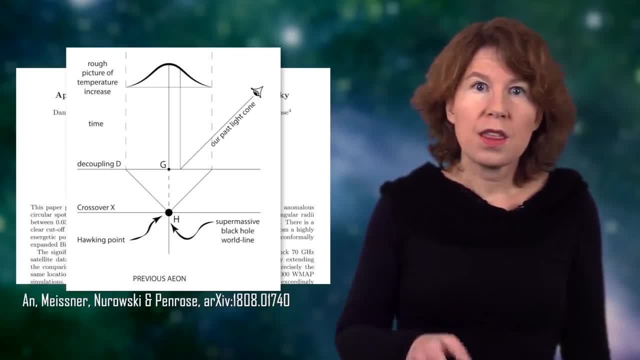 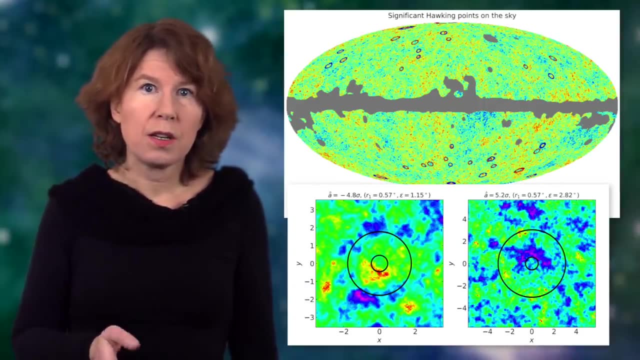 some rings around it in the CMB, And these Hawking points are actually there. It's not only Penrose and his people who have found them in the CMB. The thing is, though, that some cosmologists have argued they should also be there in the 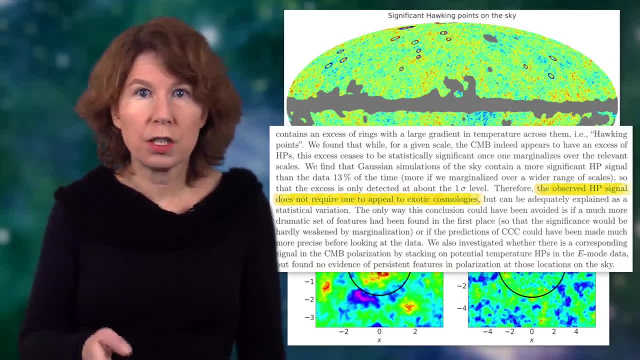 most popular model for the early universe, which is inflation. So this prediction may not be wrong, but it's maybe not a good way to tell Penrose's model from others. Penrose also says that this conformal rescaling requires that one introduces a new field, which 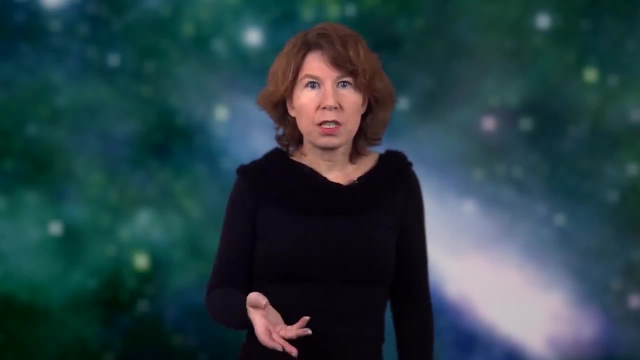 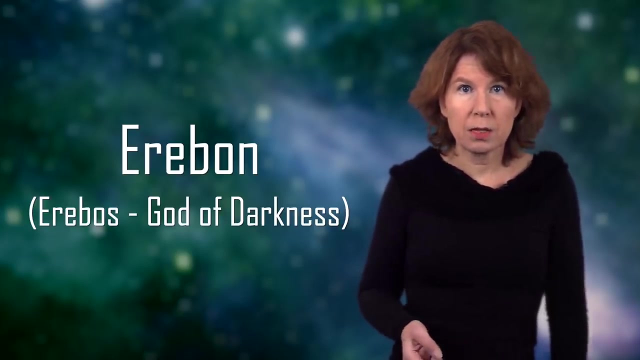 gives rise to a new particle. He has called this particle the Erebon, named after Erebus, the god of darkness. The Erebons might make up dark matter. They are heavy particles with masses of about the Planck mass, so that's much heavier. 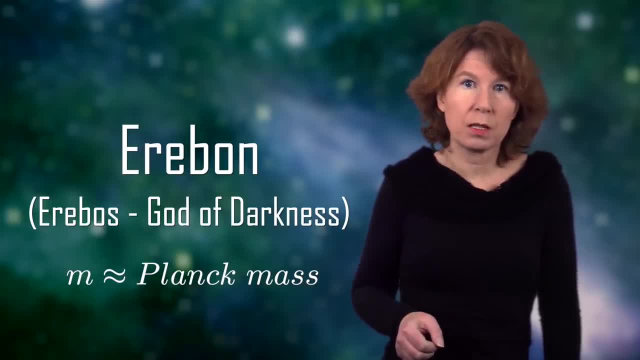 than the particles astrophysicists typically consider for dark matter. But it's not ruled out that dark matter particles might be so heavy, And in fact there is no doubt about it. Indeed, other astrophysicists have considered similar particles as candidates for dark 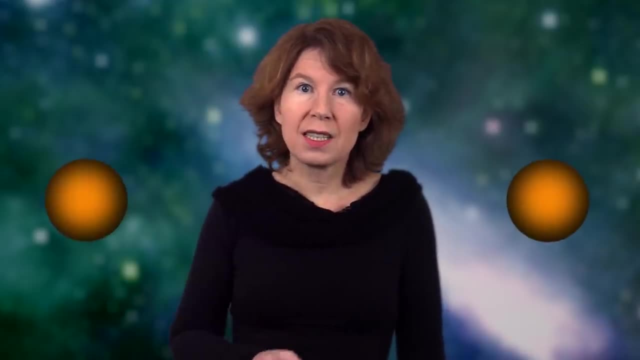 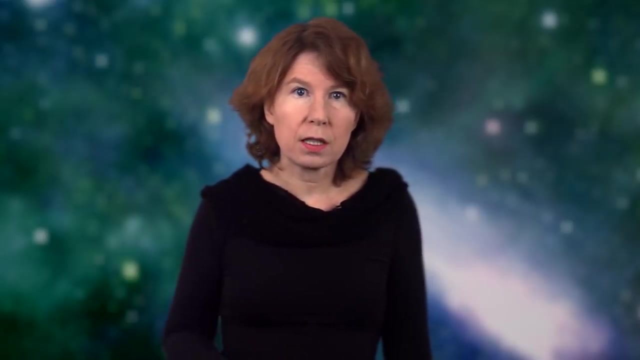 matter, Penrose's Erebons are ultimately unstable. Remember, you have to get rid of all the masses at the end of the eon to get to conformal invariance. So Penrose predicts that dark matter should slowly decay. That decay, however, is so slow that it's hard to test. 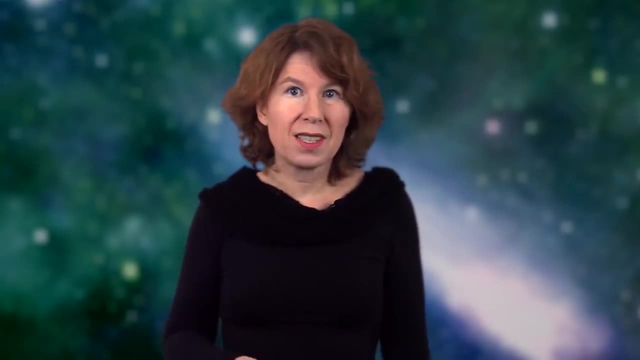 He has also predicted that there should be rings around the Hawking points in the CMB-B modes, Something that the BICEP experiment was looking for, But those too haven't been seen So far. Okay, so that's my brief summary of conformal cyclic cosmology. 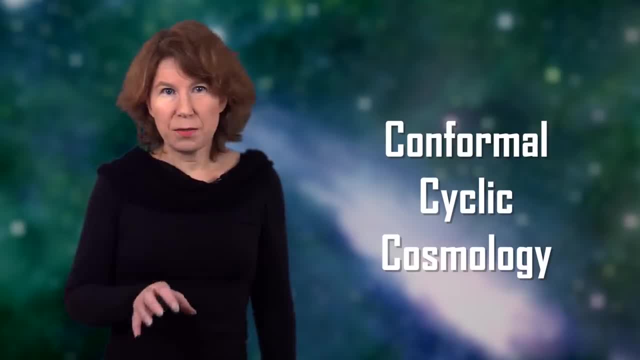 Now, what do I think about it? Mostly, I have questions. The obvious thing to pick on is that actually the universe isn't conformally invariant and that postulating all Higgs bosons disappear or something like that, is rather ad hoc. But this actually isn't my main problem. 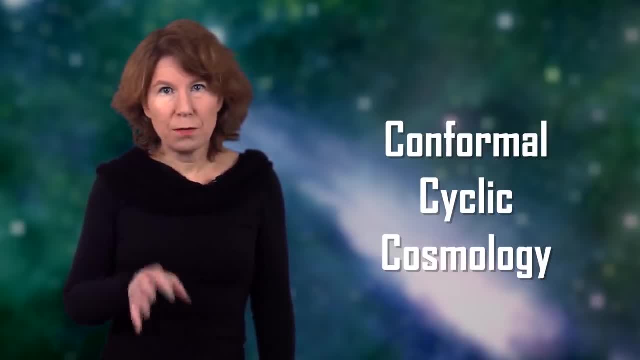 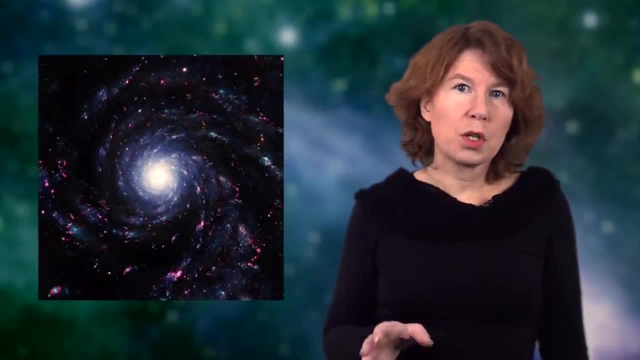 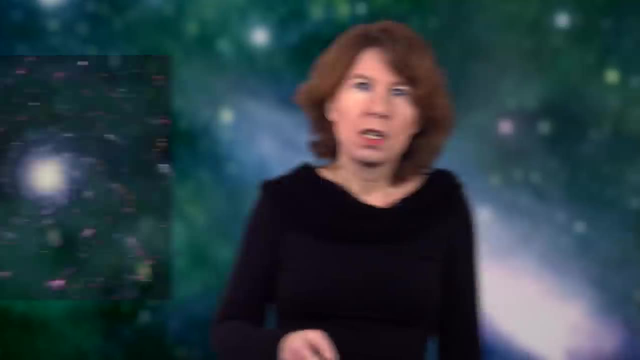 Maybe I've spent too much time among Parkinsons, But I've seen far worse things: Unparticles anybody. One thing that gives me headaches is that it's one thing to do a conformal rescaling mathematically. Understanding what this physically means is another thing entirely. 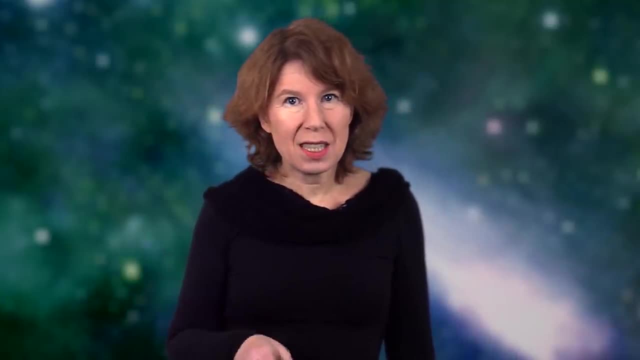 You see, just because you can create an infinite sequence of eons doesn't mean the duration of any eon is now finite. You can totally glue together infinitely many, infinitely large spacetimes if you really want to. Saying that time becomes meaningless doesn't really explain to me what this rescaling physically. 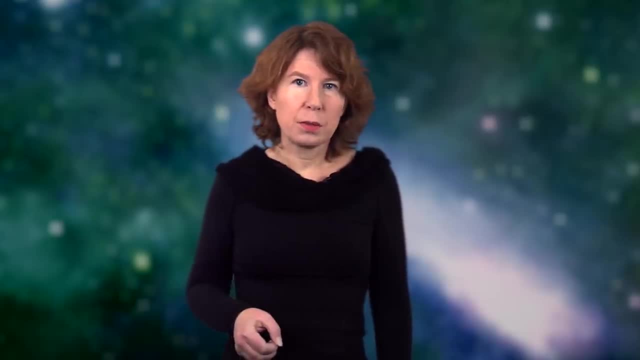 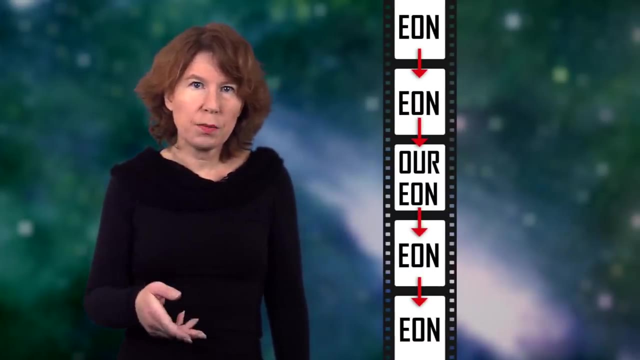 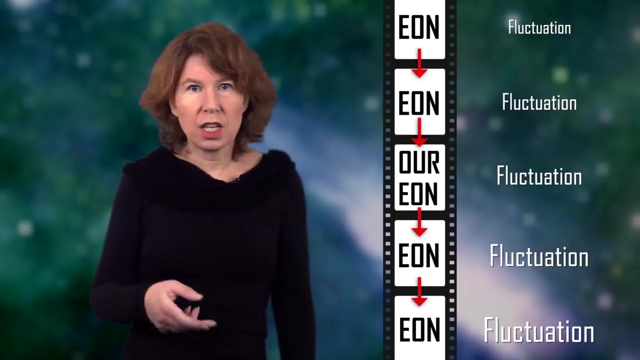 does. Okay, but maybe that's a rather philosophical misgiving. Here's a more concrete one. If the previous eon leaves information imprinted in the next one, then it isn't obvious that the cycles repeat in the same way. Instead, I would think they will generally end up with larger and larger fluctuations. that will pass on larger and larger fluctuations to the next eon, because that's a positive feedback. If that was so, then Penrose would have to explain why we are in a universe that's special for not having those huge fluctuations. Another issue is that it's not obvious you can extend these cosmologies back in time. 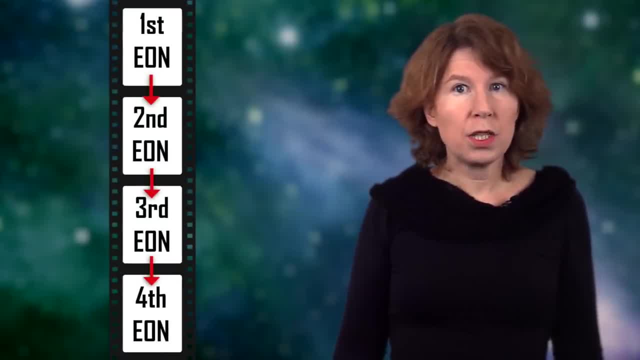 indefinitely. This is a problem also for eternal inflation. Eternal inflation is eternal really only into the future. It has a finite past. You can calculate this just from the geometry. In a recent paper I wrote that the eon is a finite past. 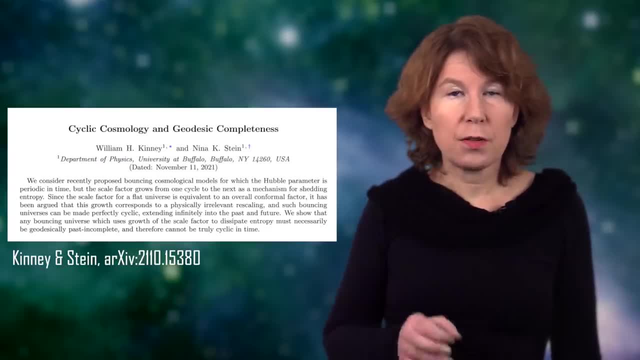 In a recent paper, Kinney and Stein showed that this is also the case for a model of cyclic cosmology put forward by Eos and Steinhardt. The cycle might go on infinitely, alright, but only into the future, not into the past. It's not clear at the moment whether this is also the case for conformal cyclic cosmology. I don't think anyone has looked into it. Finally, I'm not sure that CCC actually solves the problem it was supposed to solve. Remember, we are trying to explain the power of the eon. 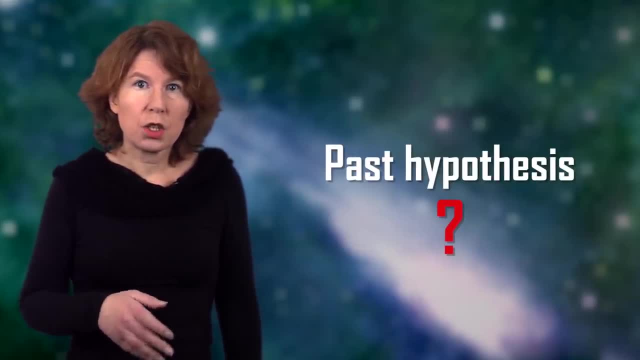 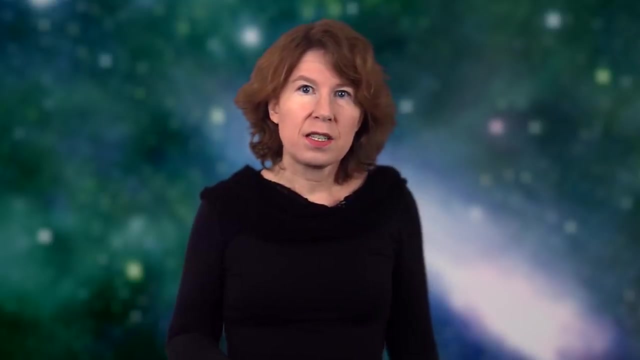 But a scientific explanation shouldn't be more difficult than the thing you're trying to explain, And CCC requires some assumptions about the conformal invariance and the error bonds. that, at least to me, don't seem any better than the past hypothesis. Having said that, I think Penrose's point that the wild curvature in the early universe 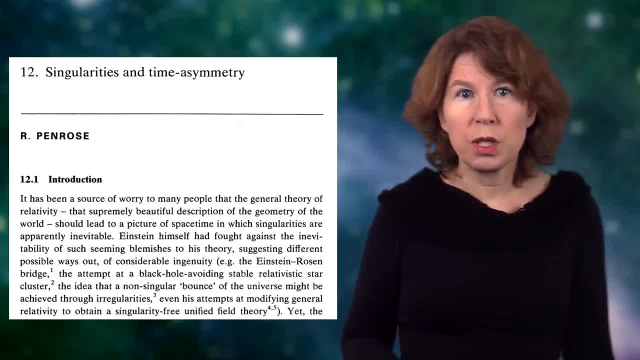 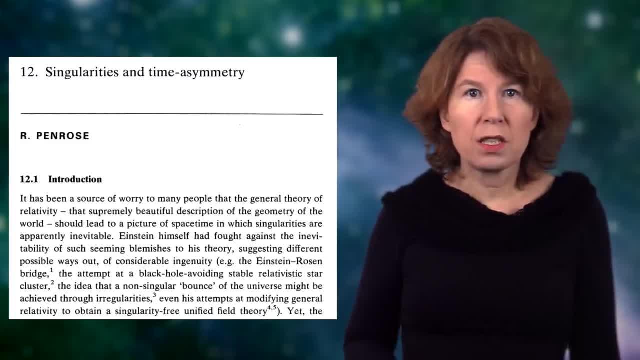 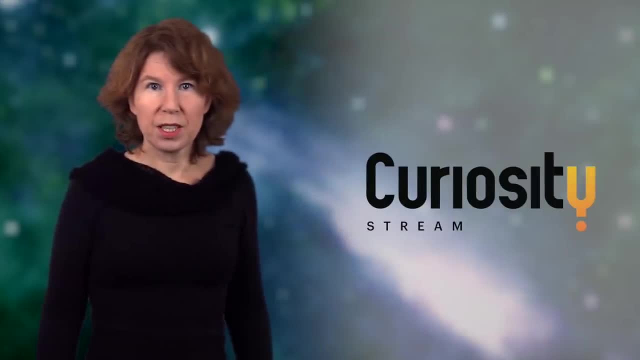 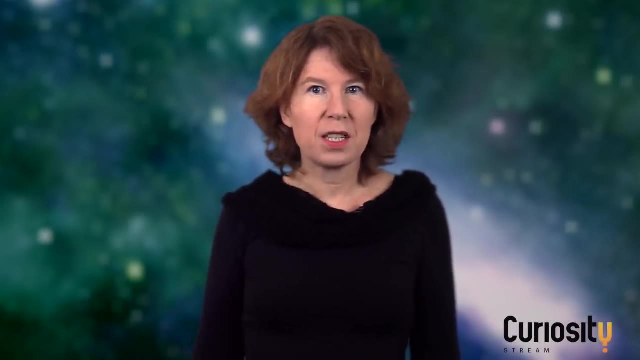 attention. This video was sponsored by Curiosity Stream. YouTube is a great place for some things. For example, from me you get the brief summaries on recent scientific topics, But sometimes brevity is not what you want. Sometimes you want a professionally made, full-length documentary. 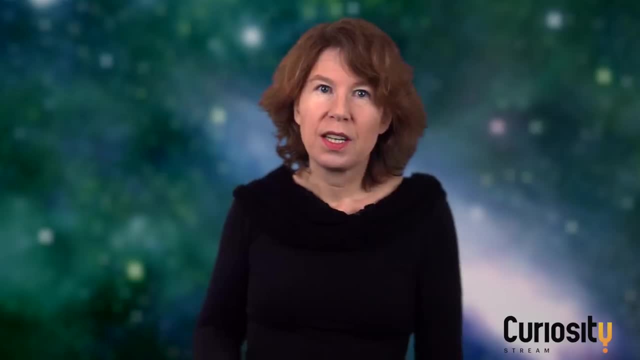 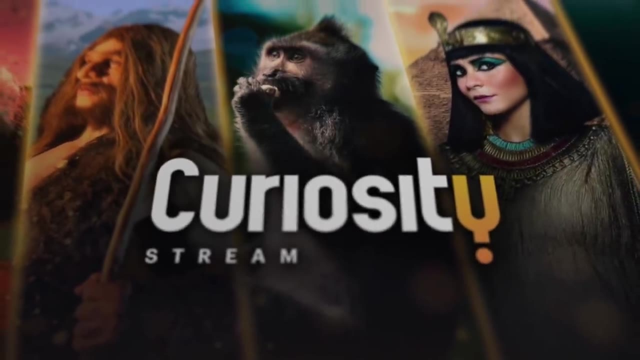 Something that will entertain you as much as it will educate you. If you like that too, you should really check out Curiosity Stream. Curiosity Stream has thousands of movies and shows about physics, space, medicine, technology, history, everything really.